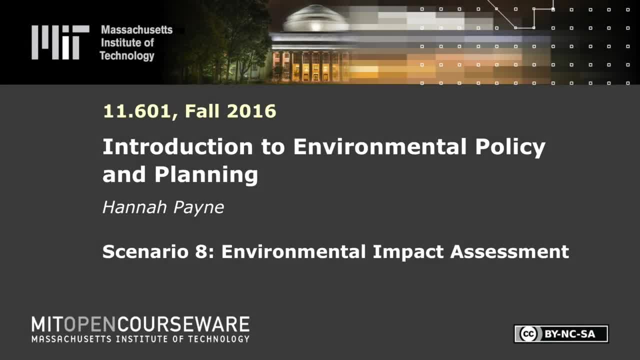 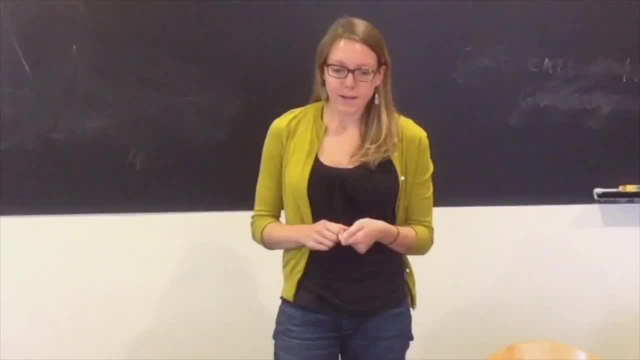 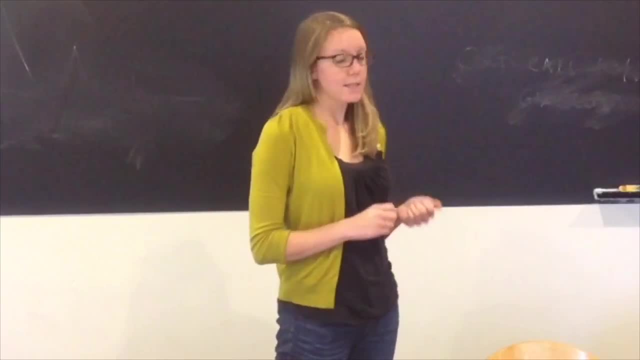 I convene this meeting because I believe that the review is limited as it stands now and, in order for the environmental impact assessment to be effective, it needs to consider a number of other alternatives in order to provide a larger scope for the project impacts both. 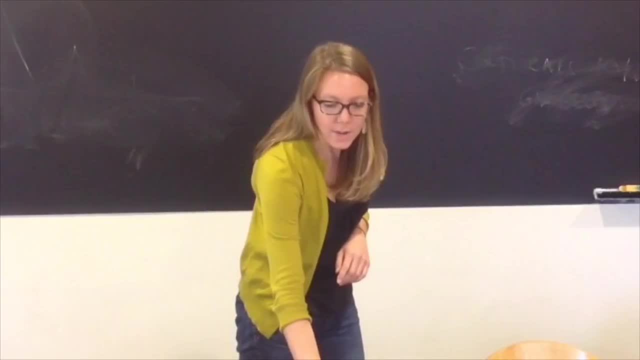 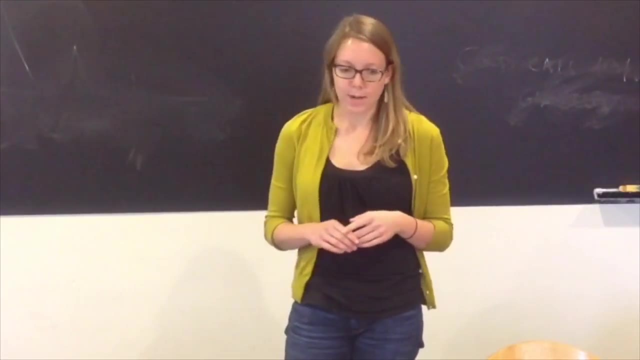 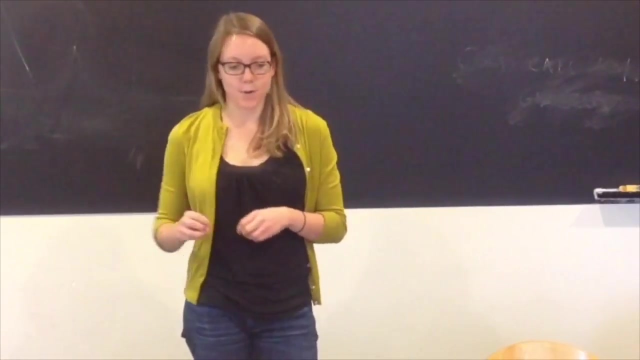 positive and negative. The draft environmental impact assessment as it stands now only considers the number of turbines, the location of the turbines and a very limited no-build option. This alternatives analysis fails to create a clear vision of the situational context of the project. In this presentation, I will be discussing ways in which we can revise. 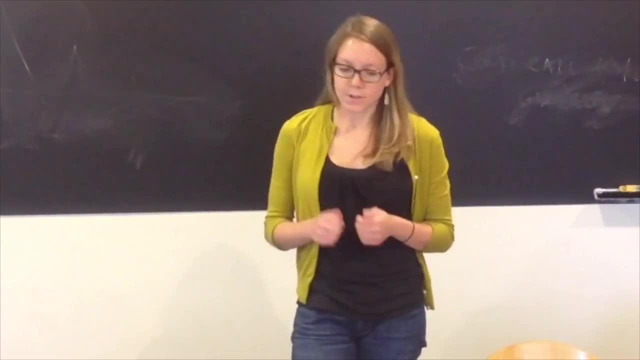 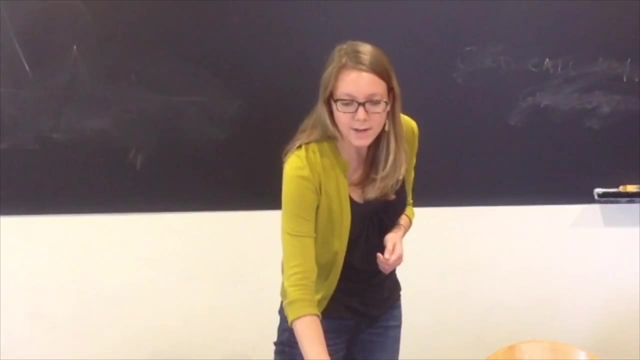 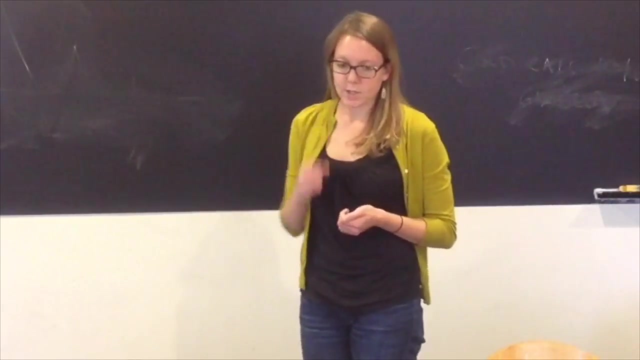 the environmental impact assessment so that it better evaluates all alternatives and will provide arguments for why it is necessary to spend the time and money to do so. First, we need to define the goal of the project if we are to effectively evaluate alternatives and consider alternative approaches. Alternatives analysis should paint a picture of the multitude 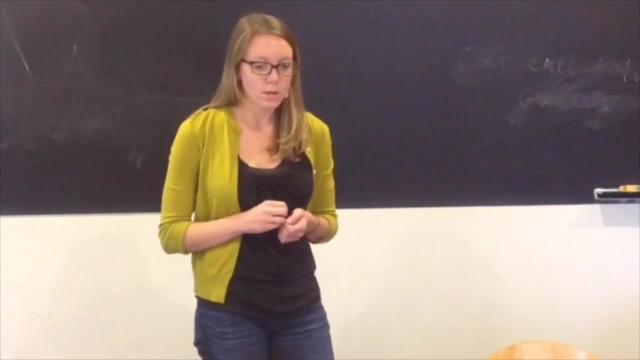 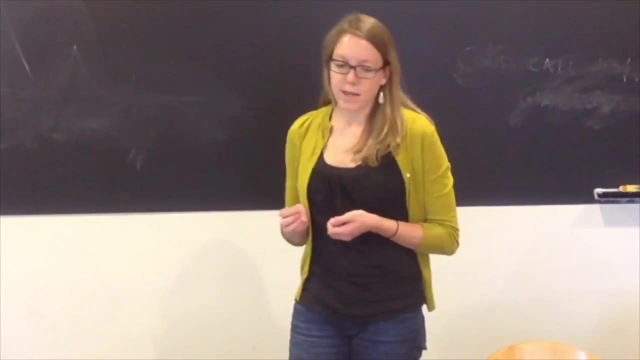 of options available to reach this goal. I believe that the goal of the project is to provide energy for the growing electricity demand in the region. Studies have shown that new energy facilities will need to be built within the next 15 years to meet this growing 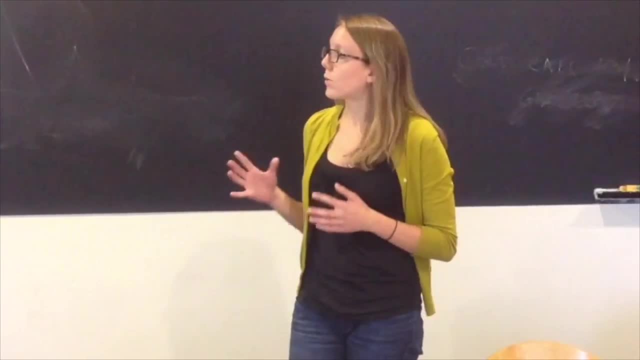 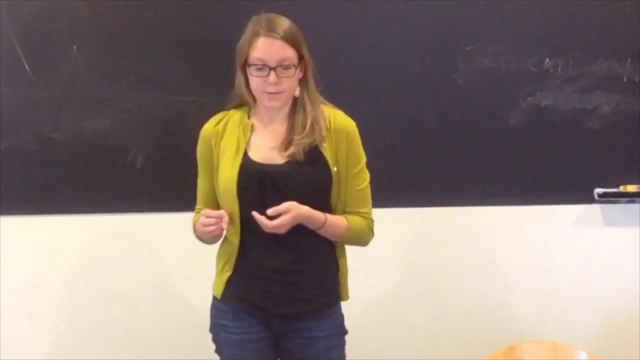 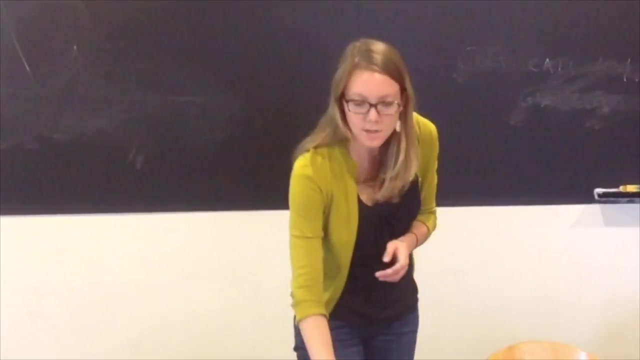 demand. We should use this goal to frame the project evaluation. Setting a clear goal at the beginning helps to consider better alternatives. It is necessary to take a step back and to see the project and its impacts in the larger context. If we all agree that the goal is. 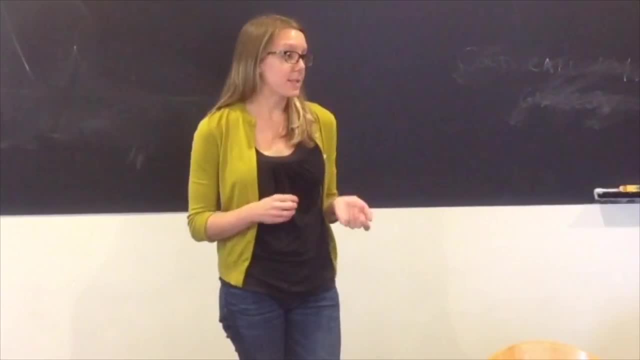 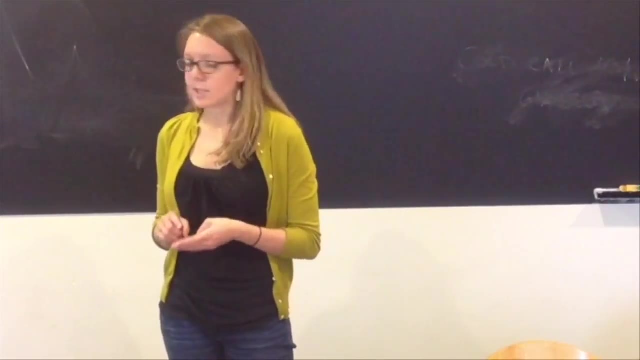 to meet the growing electricity demand. we must determine if this project is the best option and the environmental impact assessment is the way that we will do that. To do this, we need to make three major revisions to the environmental impact assessment. One we need: 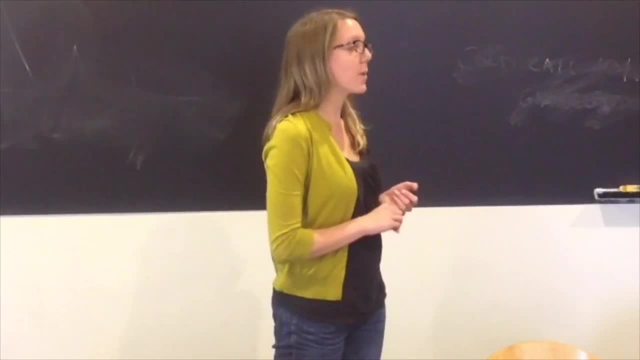 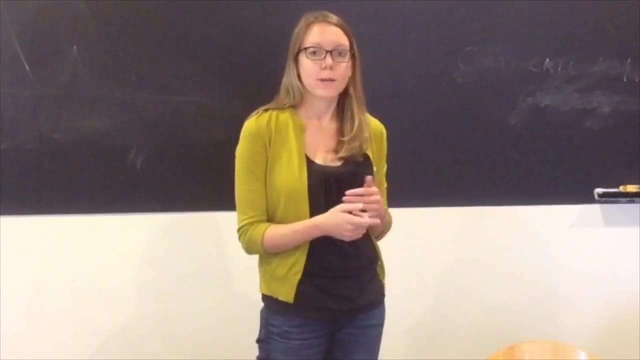 to consider alternative forms of energy. Two, we need to consider alternative forms of energy. Three, we need to consider energy production and their environmental, economic and social impacts if this plant is not to be built, If we do not build offshore wind, will we? build wind farms on land, and what will the land use impacts of that be? Will we need to build a natural gas plant to meet demand, or is solar an option? We need to really consider the greater alternatives. It will be difficult to do a full environmental impact assessment. 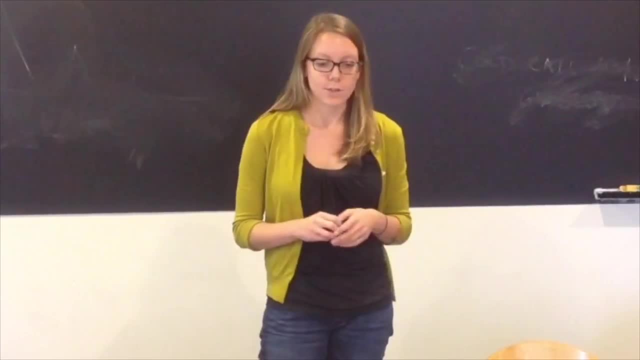 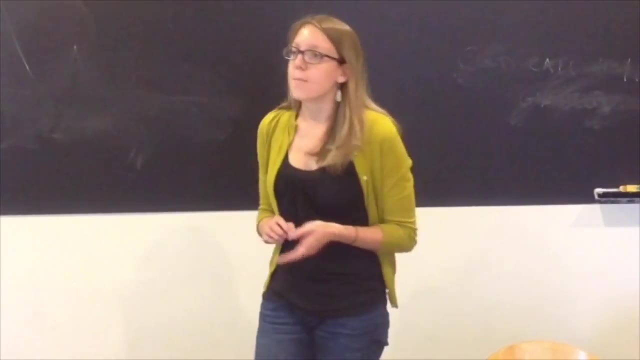 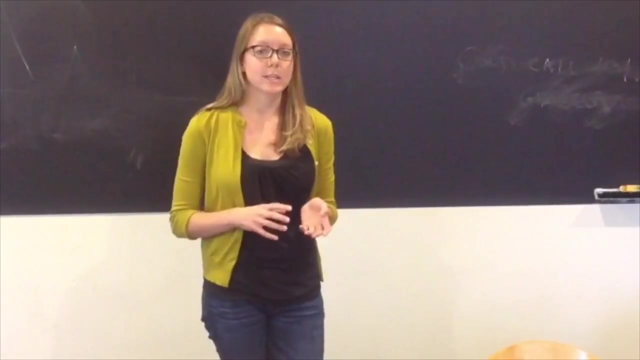 of all of these theoretical alternatives, We can pick a few items to focus on, but we will focus on, for instance, carbon emissions or land use. Second, we need to consider the impacts of wildlife and coastal communities based on cumulative impacts, if this project isn't built and other clean energy projects are not built. 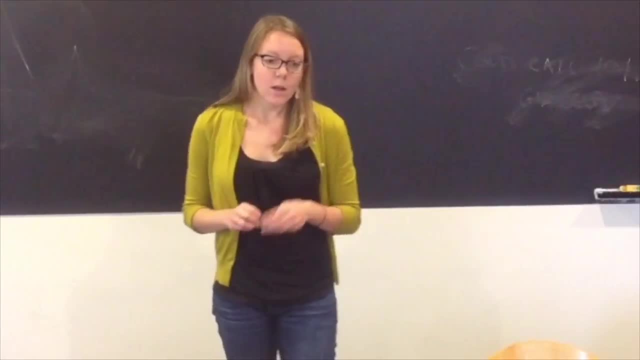 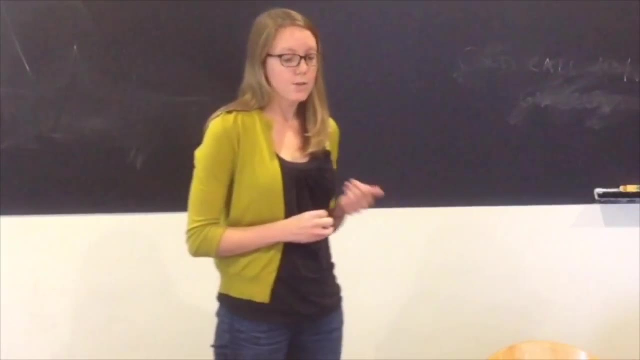 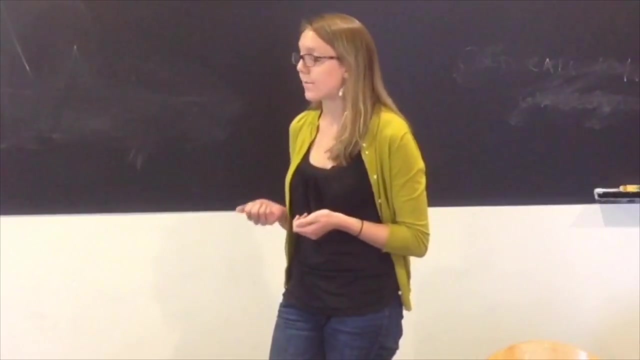 and we're not meeting our greenhouse gas emission targets. Third, if this project is perhaps the best way to meet our energy needs, then we need to consider alternative ways to mitigate the impacts. So mitigation efforts could include moving the wind farm further offshore or providing 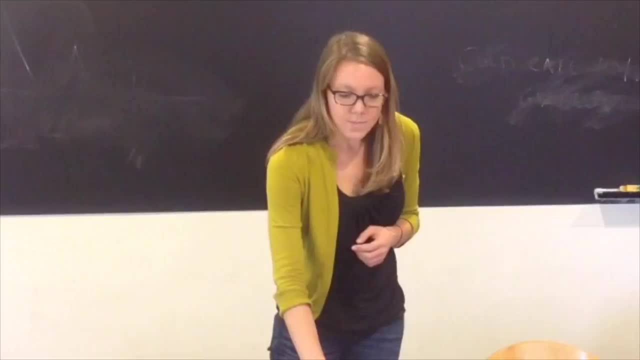 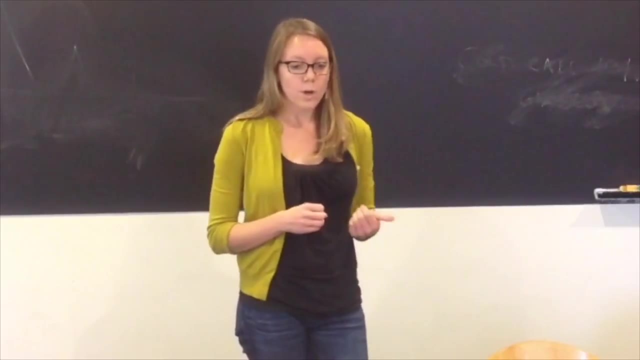 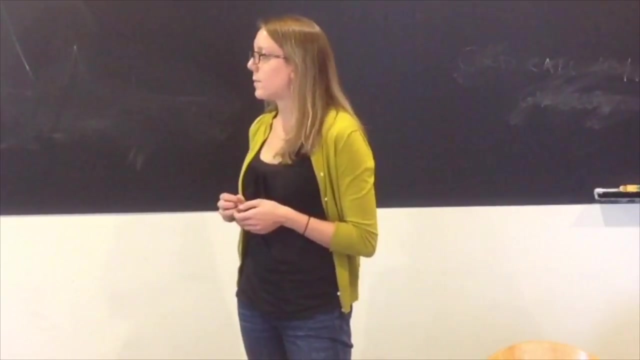 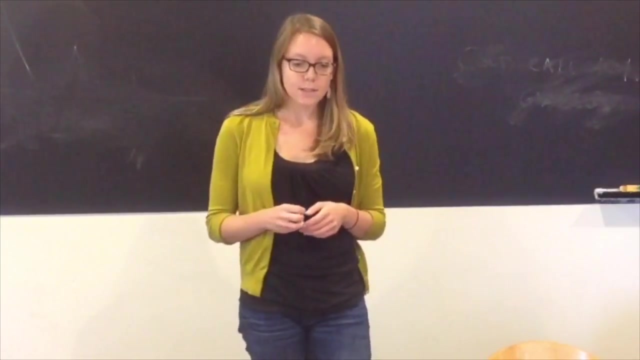 better long-term monitoring. Including all of these alternatives and a more comprehensive alternatives analysis will lead to two major benefits. One, it will increase the opportunity for public buy-in by making a more transparent process. This is really important for complex problems like energy development. And by including more comprehensive analysis, or alternatives analysis, the project 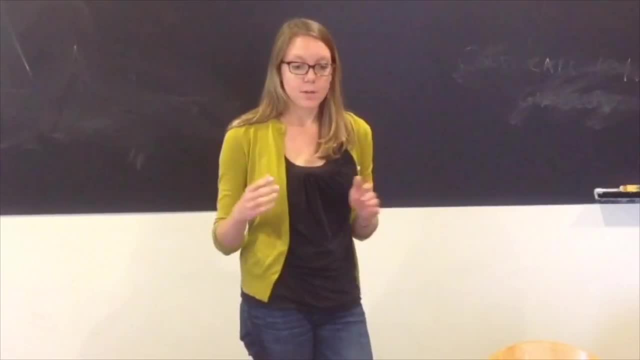 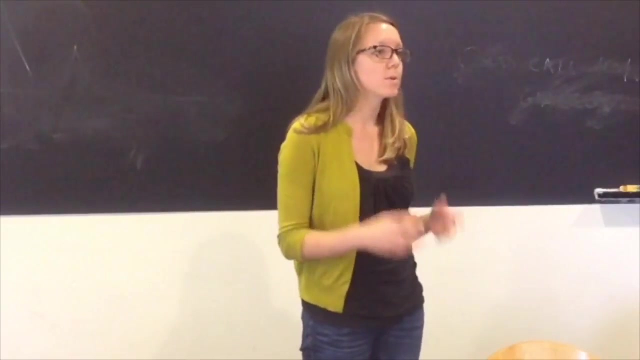 will be less likely to be fought later on because the public will be better able to use this document to see the decision-making process. The public will see that the environmental impact assessment did not just consider the impacts of the proposed pre-designed project that was already going to happen, but will 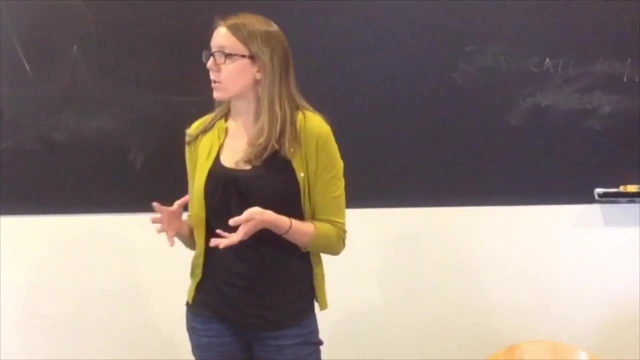 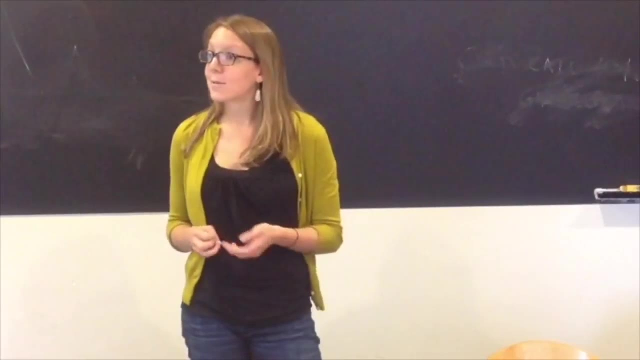 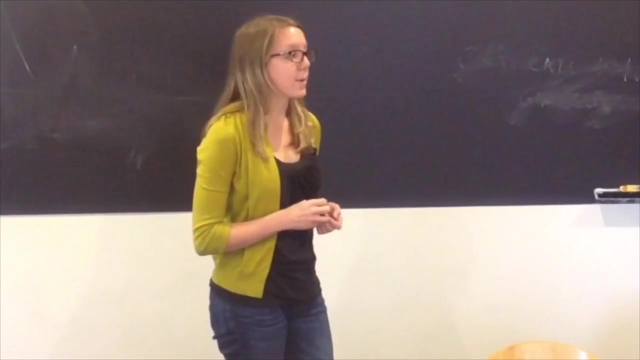 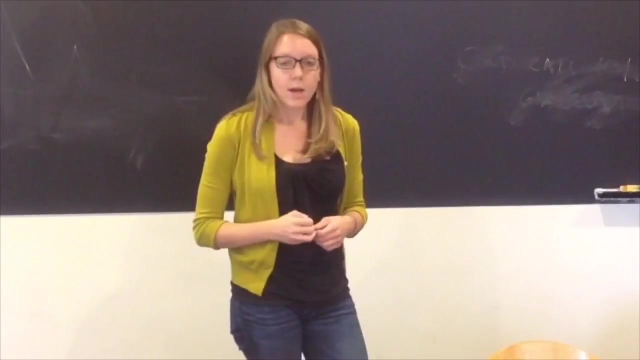 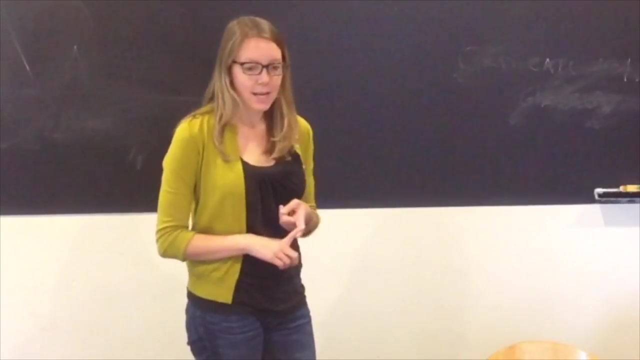 see it in a greater context. Second, because there is not much precedent for environmental impact assessment of offshore wind in the United States, we have the opportunity to set the standards for evaluation. This project will set best practices, so let's make them best practices and establish mitigation. 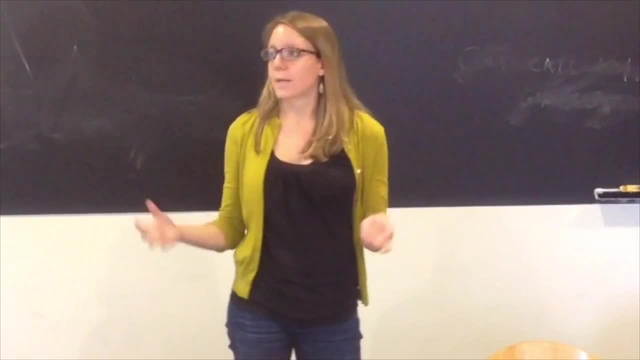 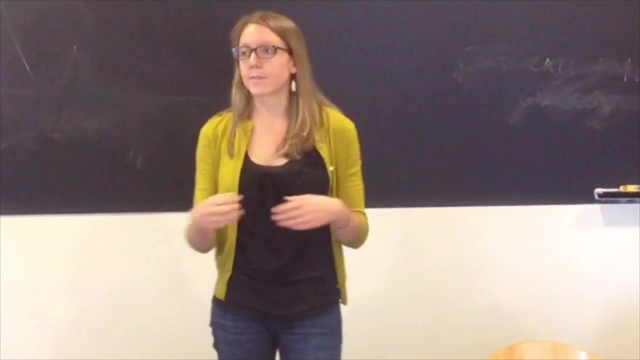 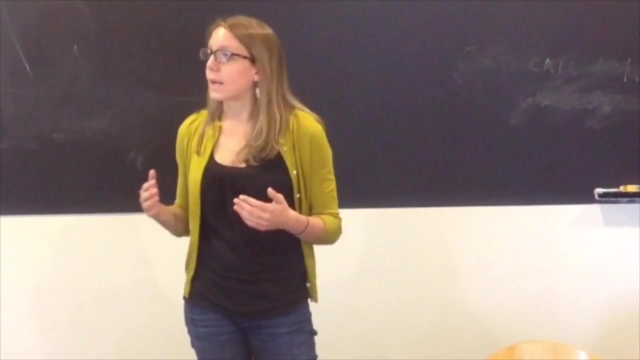 and monitoring practices, as well as the robust alternatives analysis that I have proposed. Again, we should be sure to engage the public around this alternatives analysis during the review of this draft. the comments on this draft: environmental impact assessment, so that there is public buy-in and support of the project and that the public understands.